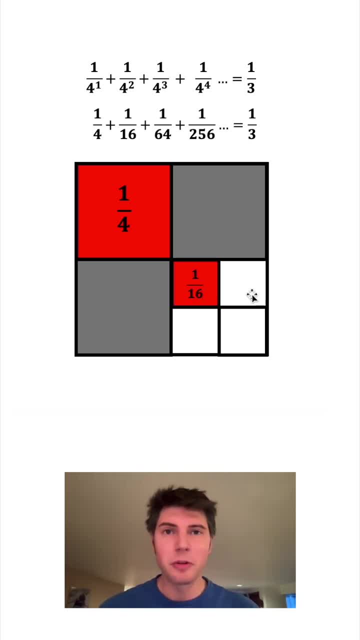 So if we color this guy red, it'll be 1, 16th of the whole square, And if we color both of these gray, we still have 1 third of all the shaded stuff is red And we can repeat the pattern again. 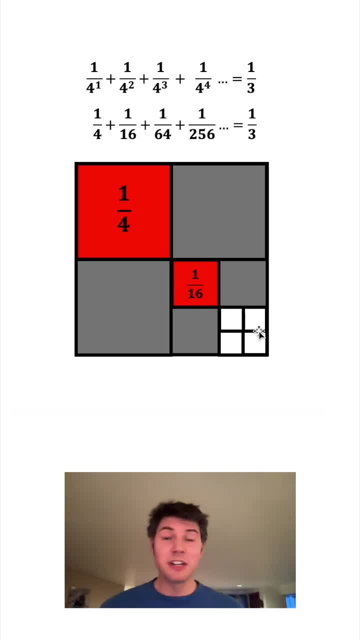 do fourths down here, and each of these is 1 64th of the entire square. If we color this guy right here red, this is going to be 1 64th of the entire square. That's going to represent this piece, right. 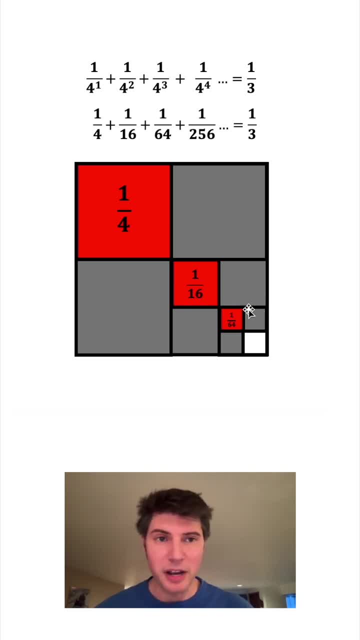 here, And then we make these gray until 1 third of everything colored here is red. So that means 1 third of everything colored here is red. And then we cut this into fourths And each of these, everything colored so far- is red. we can keep repeating new, smaller and smaller bits, and it's 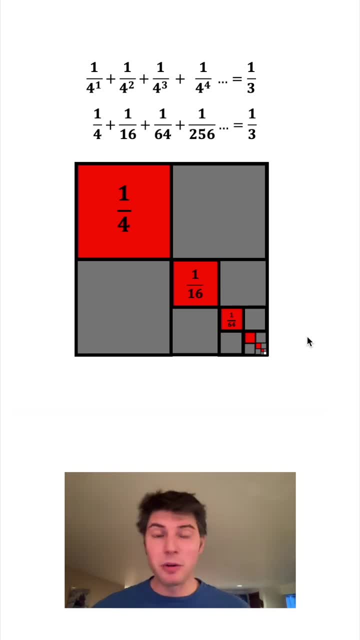 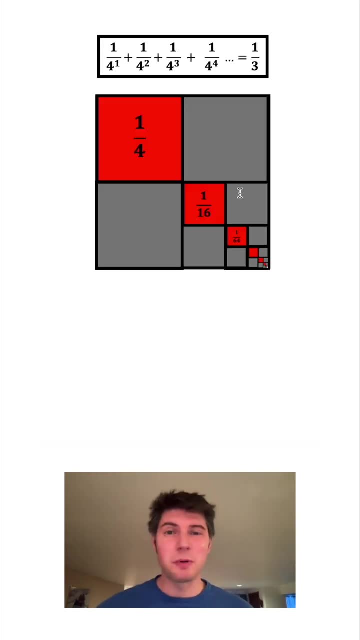 always going to keep being. one third of everything that's colored is red. that will continue indefinitely and we end up having one third of the whole thing is red. this is cool. geometrically, i'm actually convinced by this. so let's put a box around it. but we can also do it with algebra, so we take our 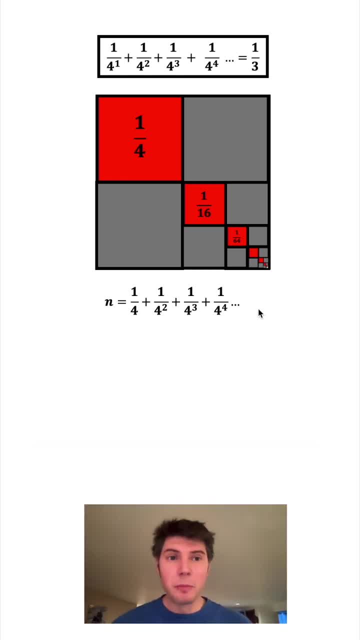 original series. it goes on forever. we set that equal to n. if we multiply both sides of the equation by four, we'll get four n on this side, and on this side each of these numerators will have a four. then we can bring down the four n. four over four is equal to one. four over four. 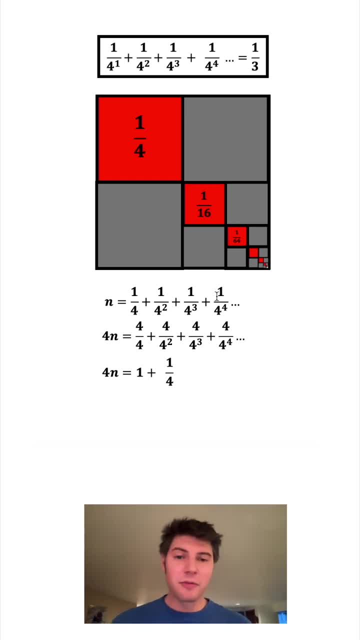 squared. well, that's going to cancel one of them, so this will just be one. fourth, then: four over four cubed- well, that'll be one over four squared. four over four to the four, that'll be one over four cubed. and that pattern is going to continue forever. this stuff in the parentheses is the.